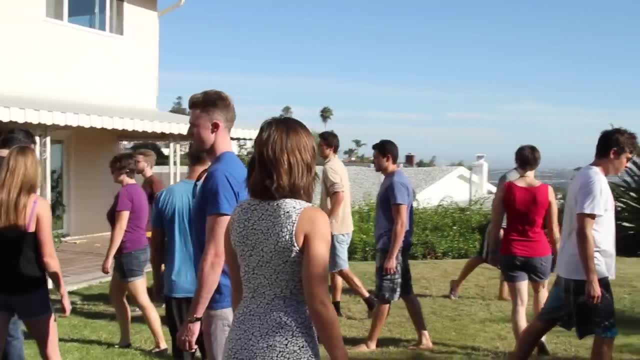 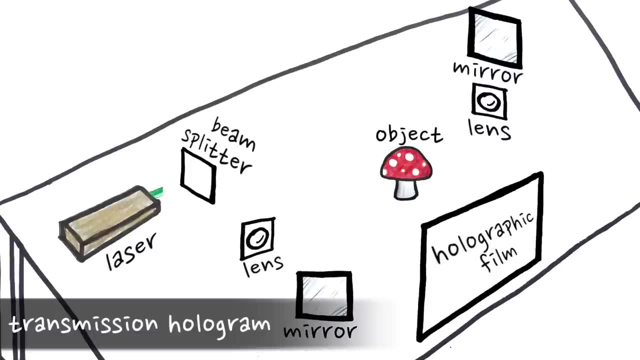 With a hologram you can move. It provides that parallax effect. Check it out. This is the setup to make one type of hologram, although the other types are similar. It starts with a laser beam which is split into two. Then both of the beams go through lenses to make them spread out. One beam: 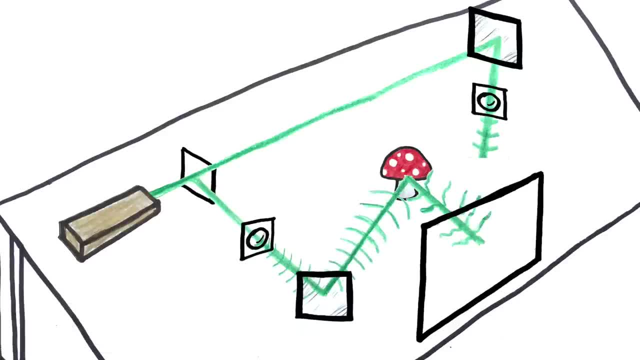 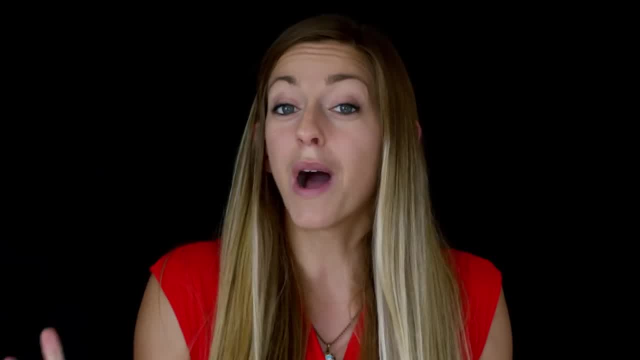 the object beam bounces off the object you're trying to image and shines onto the holographic film, while the other beam, the reference beam, goes straight there. And then, well, this is why we used lasers. Laser light looks like a laser beam, but it's not. Laser light looks like a laser. 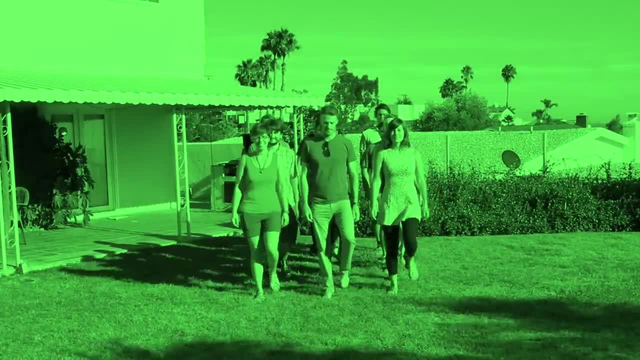 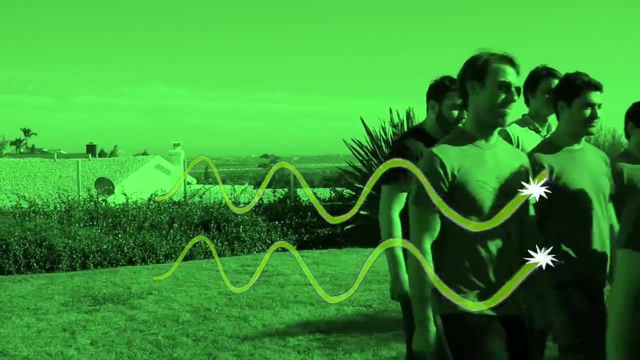 beam, but it looks very different from white light. It's all going in the same direction, it all has the same wavelength and it's coherent, meaning all the light waves are in phase or in unison. This is so key to making holograms In cases where two coherent laser beams meet. 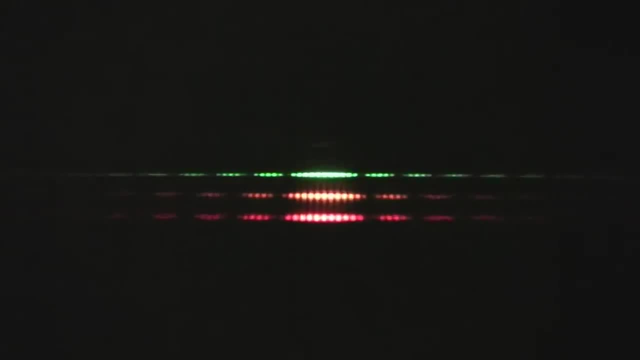 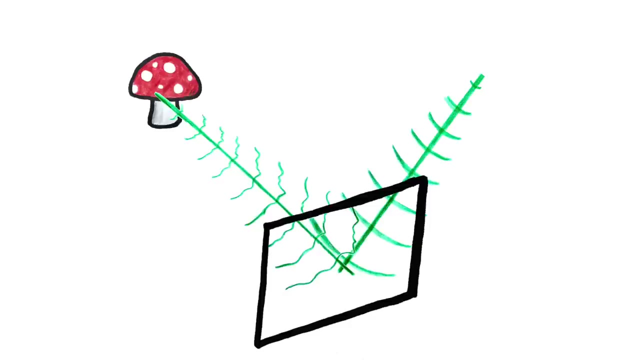 they can create regular striped interference patterns like this. In our case. the reference beam is a coherent beam, though the object beam is not. Still when they meet they also create an interference pattern. But especially if you're using a laser beam, you're going to have to. 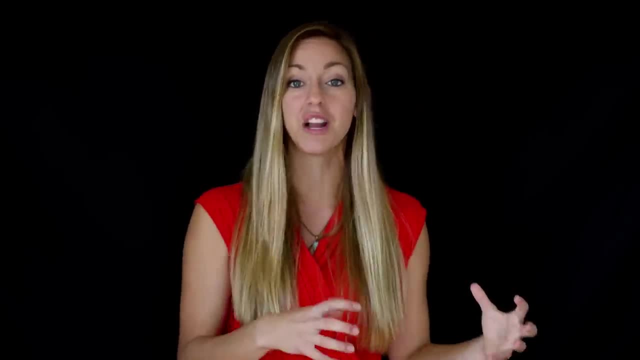 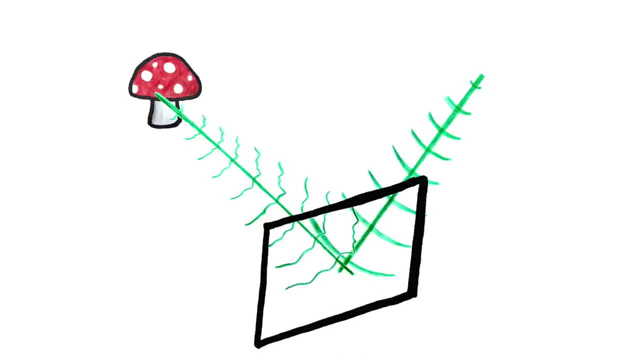 use a holographic special one that encodes the specific 3D information about the object onto the holographic film. Now we had a reference beam and an object beam, and together they created an interference pattern. A plus B equals C. What would happen if we took the interference pattern? 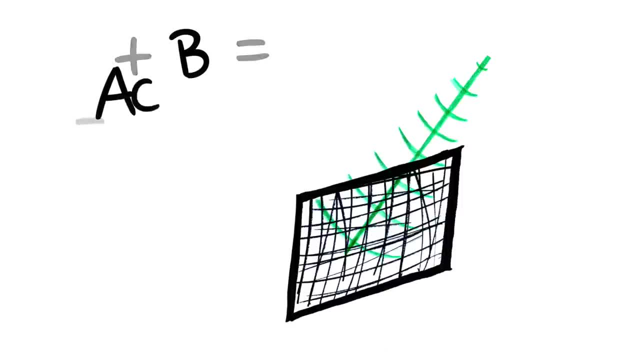 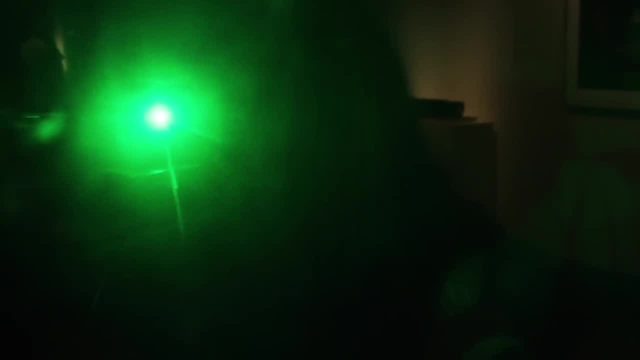 and sent the reference beam in through the back. That's kind of like C minus A. Well, that equals B, And sure enough, with this type of hologram, sending a laser beam in through the back of the film is how you get out the original hologram, And then you go back and you get a laser beam. 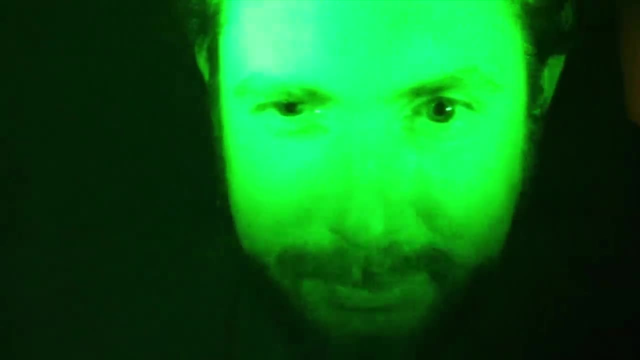 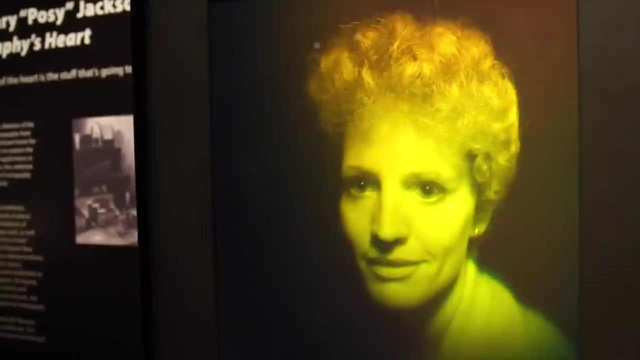 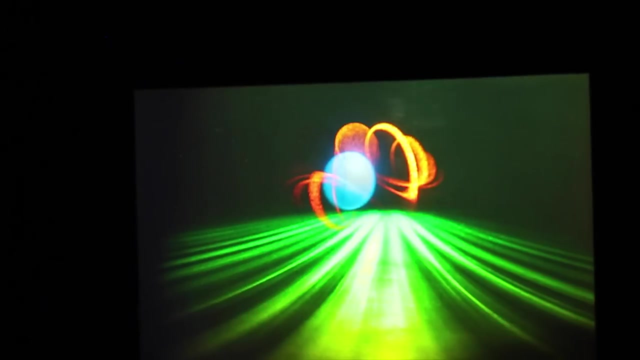 object beam. That's the same beam that was created when the laser first shined off the object. Since this reproduced beam is a perfect copy of the object beam, you can't tell whether you're looking at the light from the hologram or from the original scene, complete with motion, parallax and stereoscopic views. 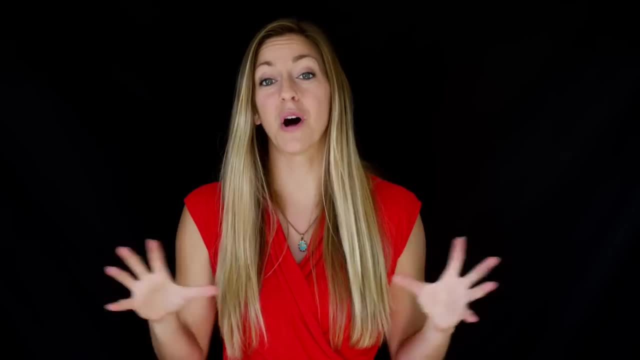 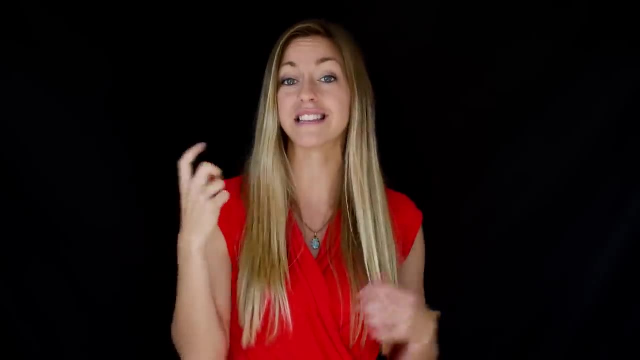 The other cool thing about holograms is that all parts of the hologram carry information about the object, so you could cut a little square of the hologram and you'd still be able to see the entire object in it. You can't do that with a photograph. Deep down, though, the holographic film is just a bunch of.